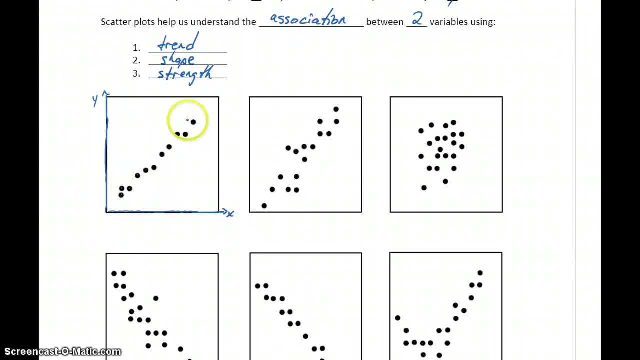 So in this case we can see that as we read the graph from left to right, our points are increasing, So we could describe the trend as an increasing trend. The shape in this case is approximately linear, because our points are following a straight line pattern, more or less. 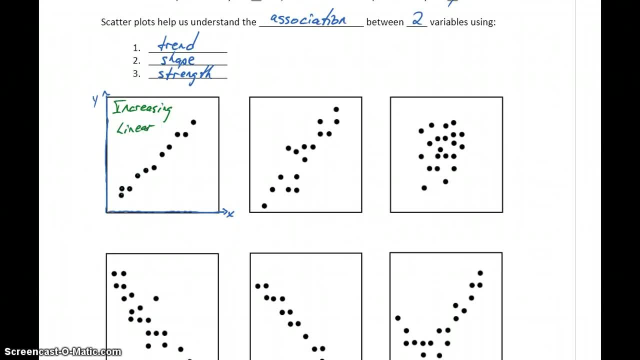 And then, in terms of strength, we want to talk about basically how close those points fit to that shape that we identified. So in this case we're saying it's a linear pattern And in this case the strength of that association seems to be very strong. 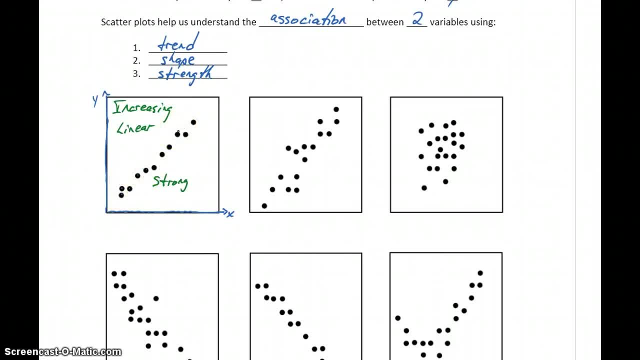 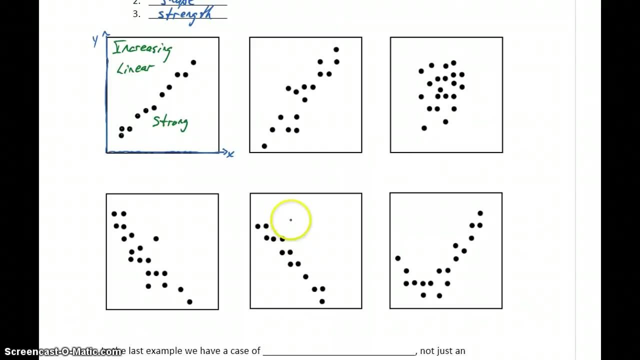 because the points closely follow that straight line pattern. So that's an example of an increasing trend. If we jump down to the second row, we have an example of a decreasing trend. So in this case our points are headed down as we read the graph from left to right. 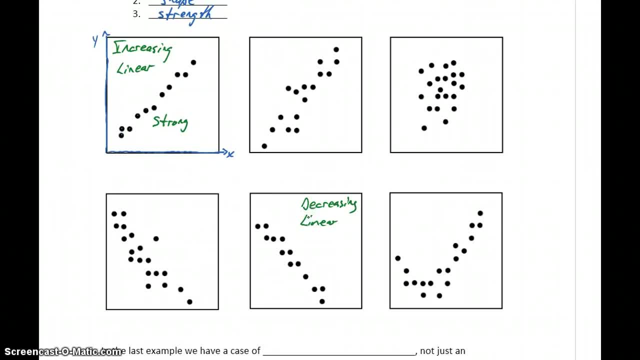 We still have a linear shape And again we have a relatively strong strength or a strong association, since again they follow pretty tightly to that straight line pattern. So other cases we might see would be in our second graph. here We still have an increasing trend. 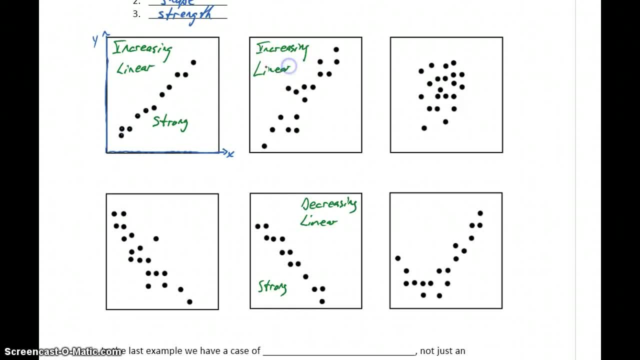 We have a linear shape But we have not necessarily a weak association, but not quite as strong because the points there's a little bit more scatter in our graph, So we might refer to this as a moderate or fairly strong association. First graph: on the second line is again a decreasing trend. 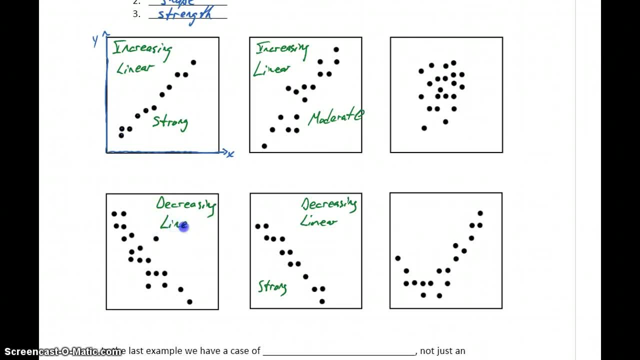 The shape is still more or less linear. And again we have more of a moderate strength to that association because our points aren't following that straight line pattern quite as closely as they did in this other example. For our last two we've got a graph here where the points are sort of scattered around. 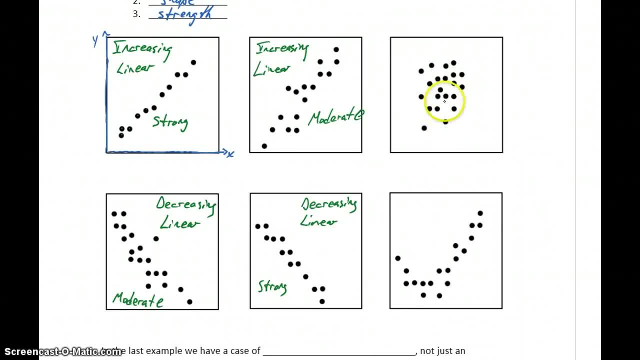 There's no particular straight line pattern, no kind of shape really occurring here. So in a case like this, we would simply say that it looks like there's no association. The points don't seem to be following that straight line pattern, seem to be following any specific pattern. They're just sort of scattered or spread around. 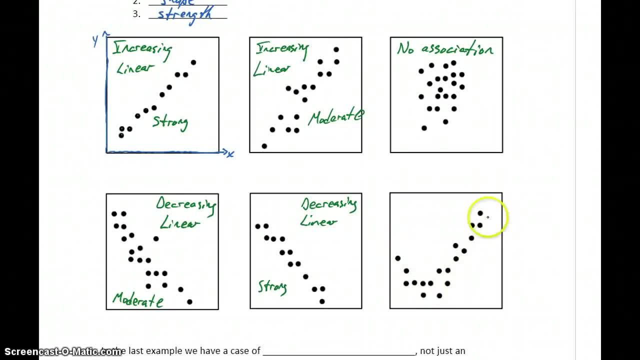 And then our last example. we still have sort of a bit of scatter, not exactly a linear pattern, but if we sort of trace the pattern that these points are going, we would trace out sort of a parabola shape. So in terms of shape we could refer to this as 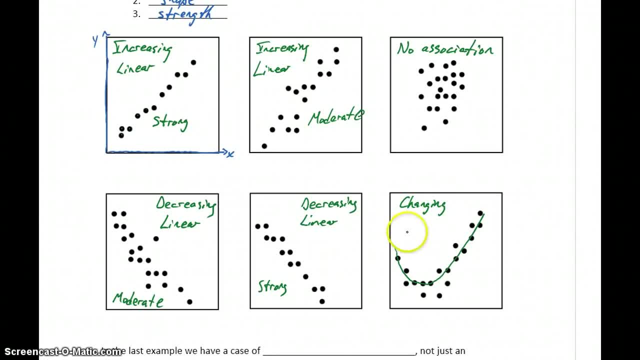 a changing shape. We could refer to the shape as a parabola or a curve, And again we've got a relatively moderately strong association. The points follow pretty closely to that pattern, but there are a few points that kind of spread away from that. 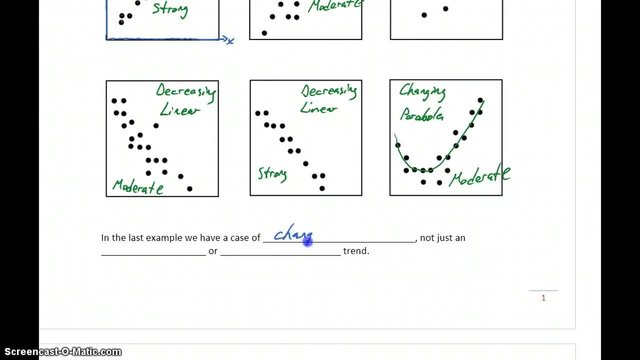 So in that last example again, what we have is a case of changing trend, Not just in the first few examples where we saw specifically just an increasing or- excuse me, increasing or decreasing trend. For our purposes, what we're going to mostly be interested in, 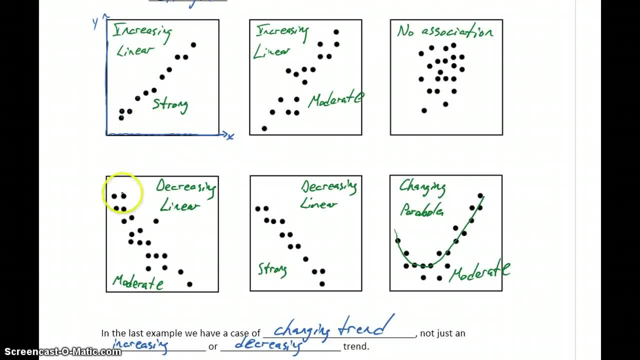 finding are variables that follow a linear shape. So either of these first four examples. there are statistical processes for looking at scatter plots and variables that follow other types of shapes, Parabolas, different types of curves, But for our purposes we're going to be mostly concerned with identifying when two variables have a linear shape. 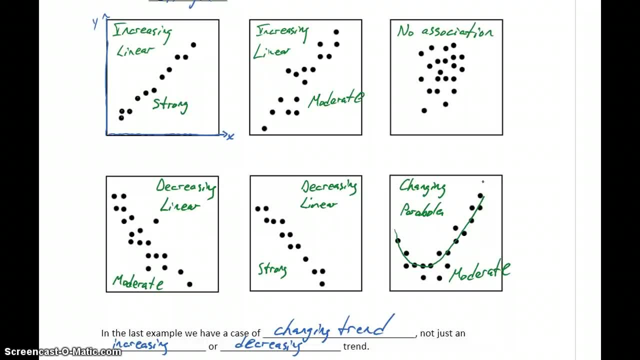 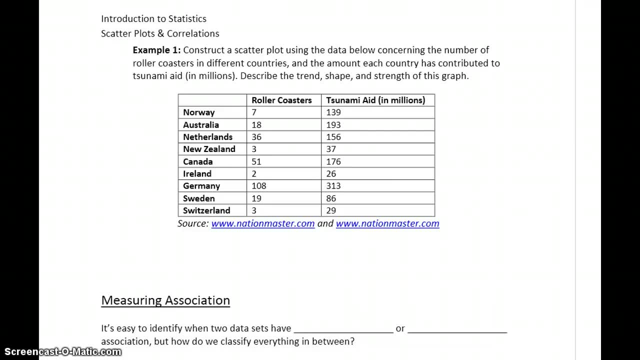 and then talking about whether that's an increasing decreasing trend and how strong that correlation is or how strong that association is. So in our first example, let's take a look at, given some data, actually constructing a scatter plot and then describing the trend, shape and strength of that graph. 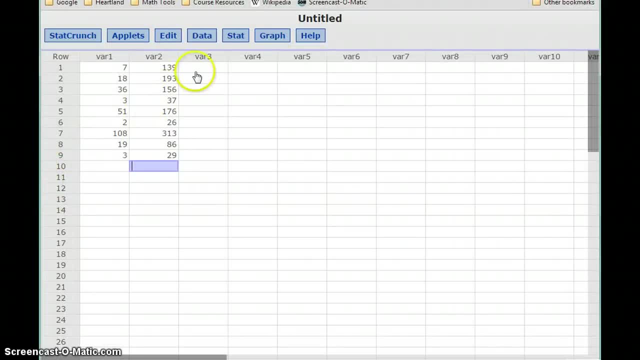 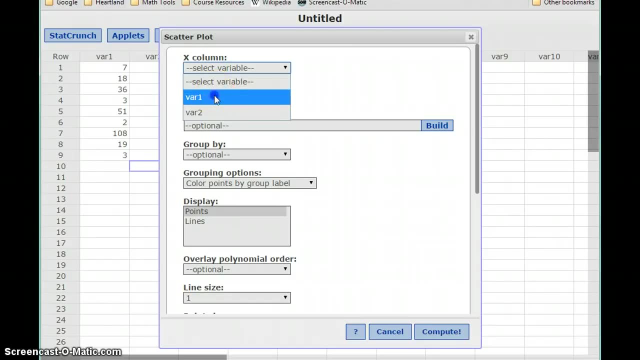 So with our data in StatCrunch, we can select graph and then scatter plot. We'll select our first variable and second variable. We have some other options here, but for now that's all we really need to indicate And click compute. That will generate this scatter plot for us.